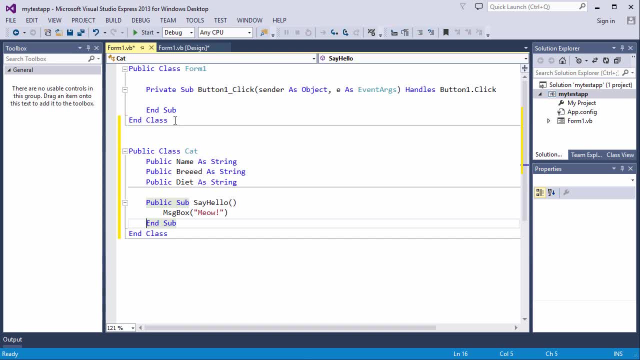 It's a procedure that outputs what a cat would say if it was saying hello. At this stage it's looking a bit silly, But bear with me for now. I'll show you something more realistic later. So here's my Cat class. 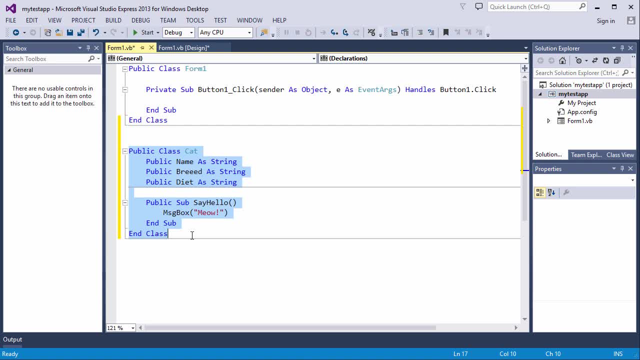 And you can see what a class is. A class is code. To be more precise, though, a class is code that defines an object, Code that can be used to create an object, So let's create an object from this class. 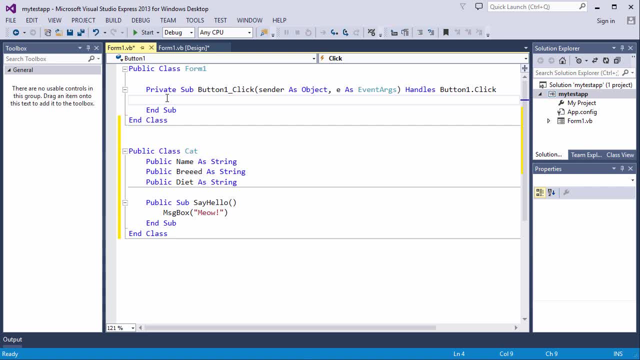 In my Forms file. I'm going to create a new object. In my Forms buttons, click event. I'm going to start by declaring a variable. Shall we say C1. And it's going to have a type of Cat. Notice, Cat is in the list of variable types now. 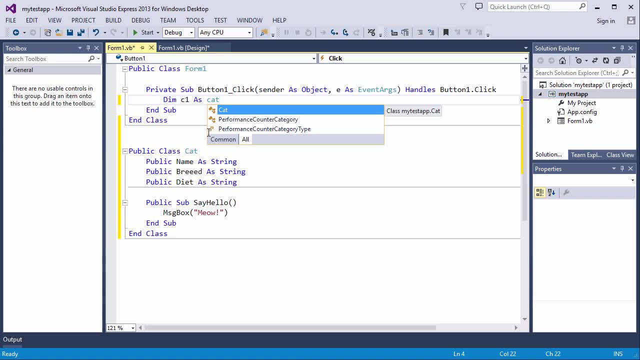 In fact, another name for a class is a type. Of course, it's not a simple type like an integer or a string, But it's a type nevertheless. Now I'm going to write a line of code To create a new Cat object. 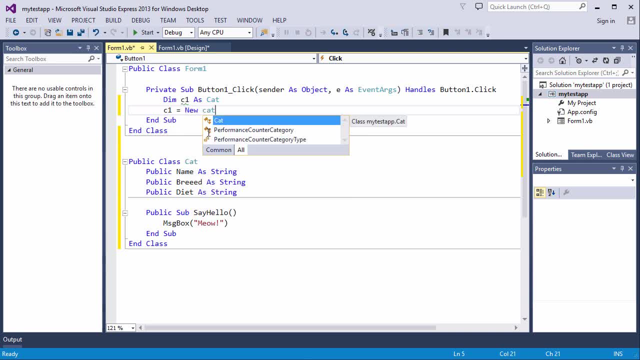 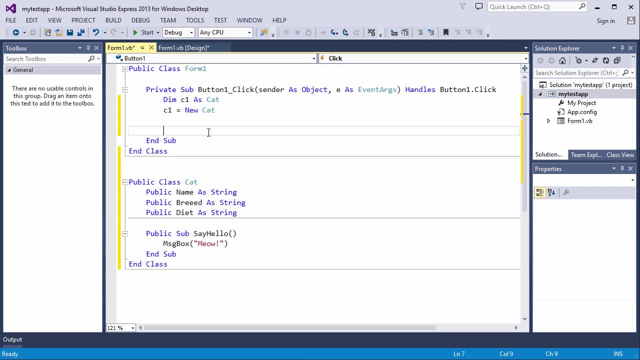 When this line of code executes, a Cat object will be created inside the computer's memory. My Cat will exist. It will come to life, if you like. Now, I'm always very careful how I use the word create when I'm talking to programmers. 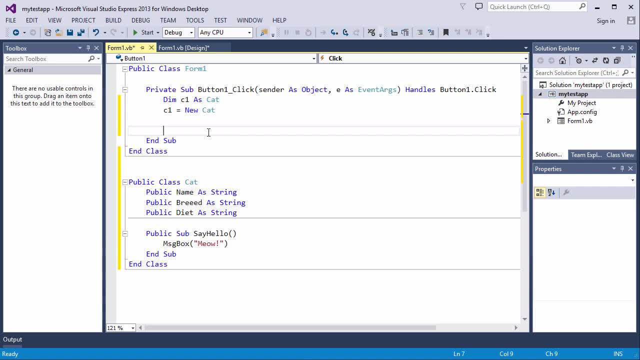 You won't ever hear me saying I'm going to create some code. I write code. In the world of OOP, the word create is used. The word create has a very specific meaning. It means to create an object from a class. 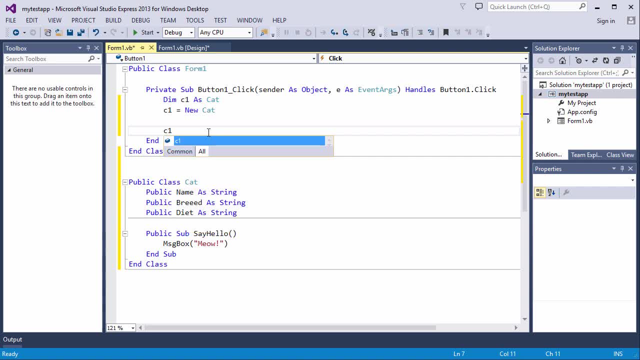 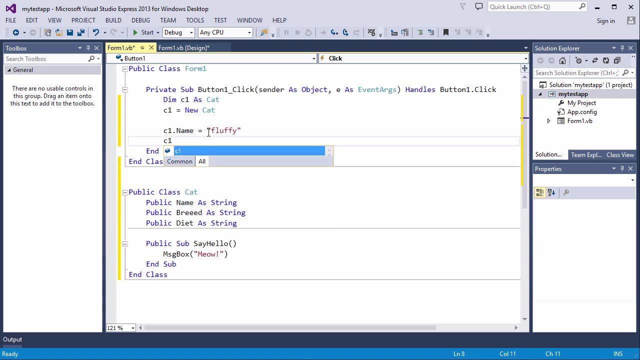 Now let's set some property values. I type C1.. And then notice the list of properties. I can select one from the list. I just use my Tab key And I'll give this Cat a name. I'll give it a breed. 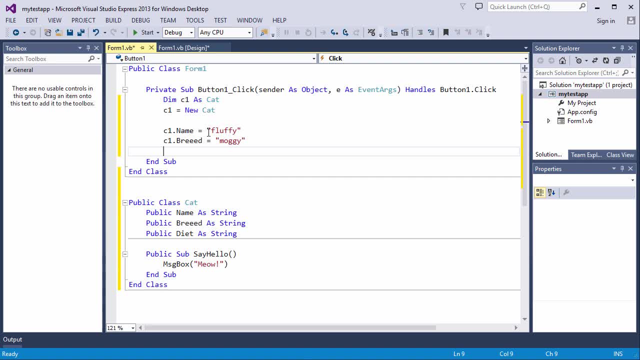 I'm not an expert on cats, so I'll go with Moggy for now. I've noticed a spelling mistake there as well. I'll have to sort that out in a second. Breed is not spelled with three E's, And let's sort out the diet as well. 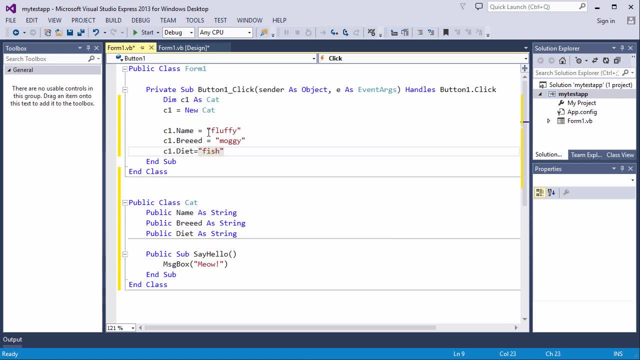 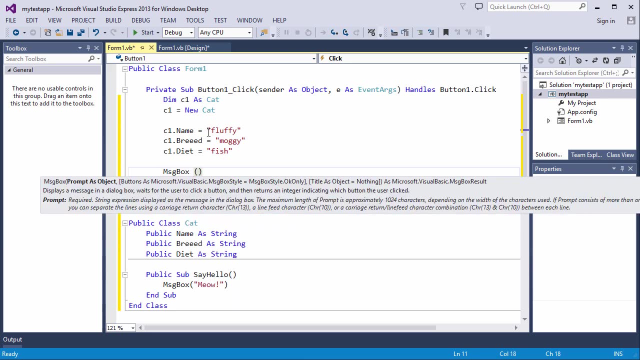 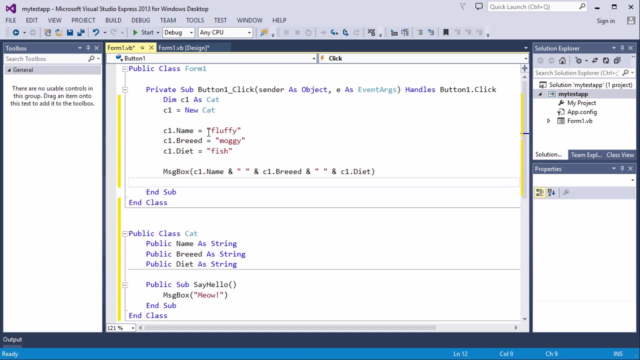 Fish. Cats love fish, don't they Notice that setting a property value is very similar to assigning a value to a simple variable? Now I'll output the values of these properties. Notice that interrogating a property value is very similar to interrogating the value of a simple variable. 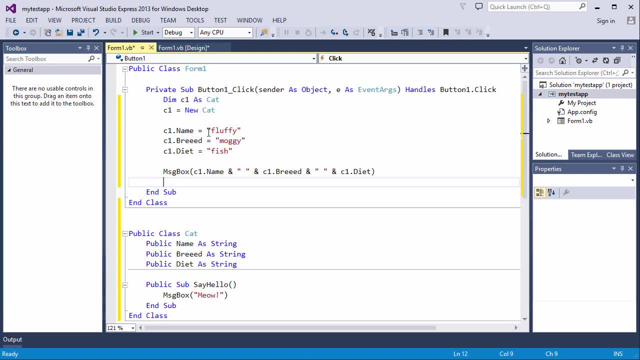 Working with properties is very intuitive. I just proceed the property names with the object name, In this case C1. Now let's write some code to call the SayHello procedure. The public procedure has become what is known as a method or a behaviour. 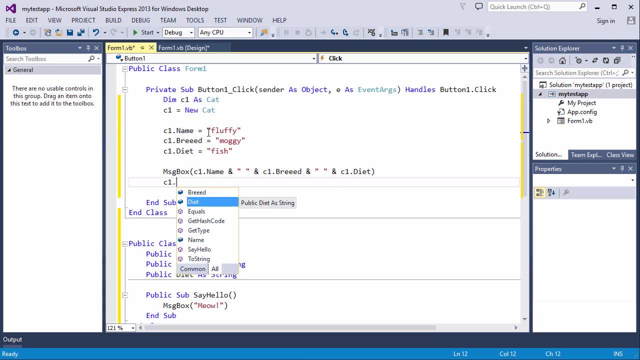 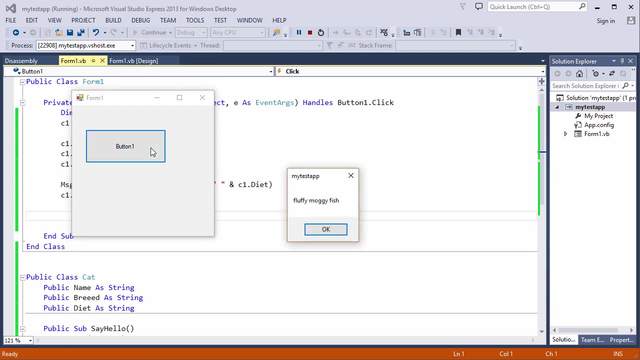 There are some other methods here which we got for free. They'll make more sense later, when I discuss inheritance. Let's just keep it simple for now, though, So let's run this code and see what happens. There are the property values that I set being output. 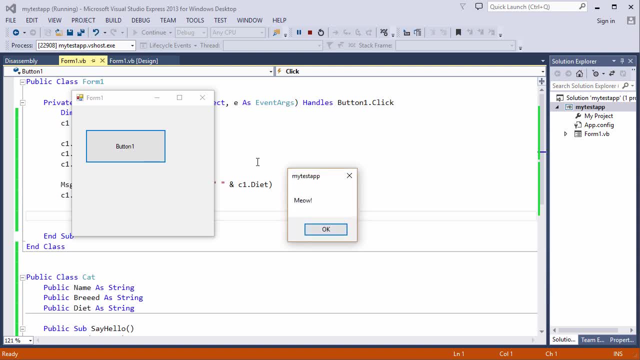 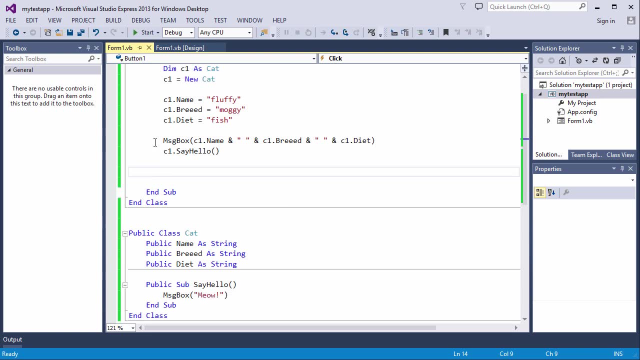 I dismiss this message. And there's the method call. Now I'm just going to fix that little problem that I had with my spelling. I'm just going to change the name of this property. Yes, I've spelled it correctly. Now, if I take a look back up here in my application, which is using the class: 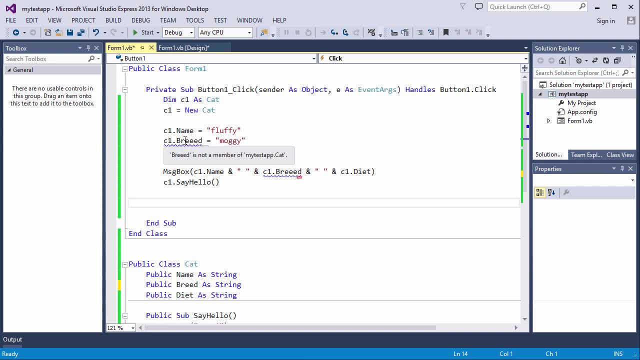 I've suddenly got some error messages, because what does it say? Breed is not a member of my test appcat. In other words, breed with three E's is not a property of a cat. So I do need to fix that now. 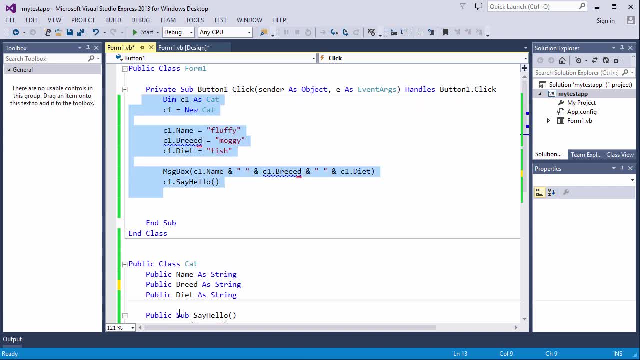 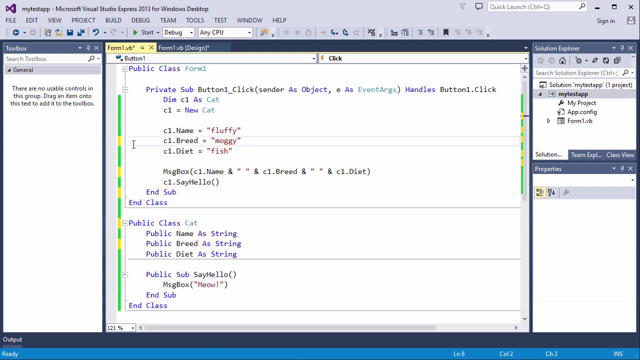 I've effectively broken this application by changing the public interface of my cat class, So let's just repair that very quickly And that should be absolutely fine again. To summarise so far, then: An object is a thing from the real world, like a person or a car or, in this case, a cat. 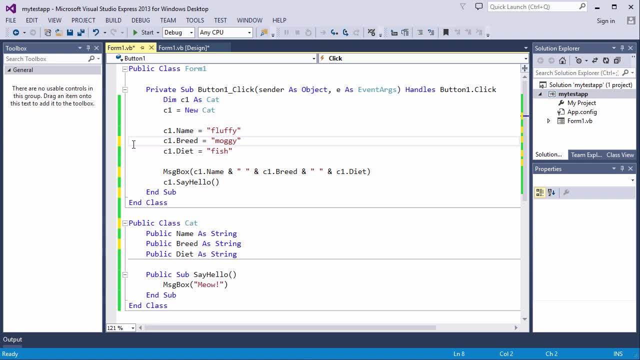 It could also be something that you can't touch, like a booking for a cinema ticket, or a bank account or a dental appointment. Nevertheless, an object is an entity from the real world that we want to store and process some data about. 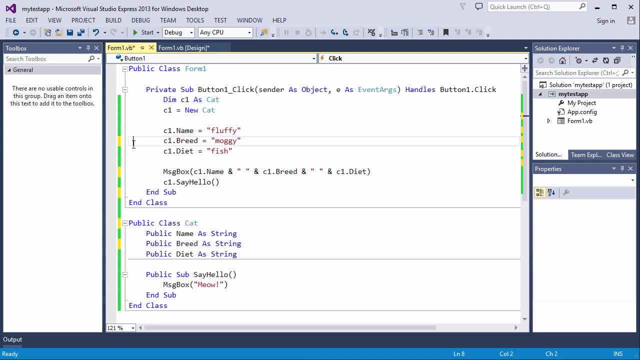 A class, on the other hand, is code. It's the code that defines a type of object. A class code defines the properties of an object. Properties are the characteristics of an object. They describe an object. They're often referred to as attributes. 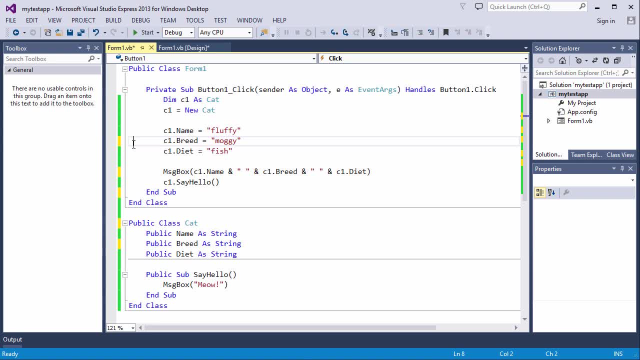 Class code also defines the methods of an object. Methods are sometimes referred to as behaviours or operations. Methods are things that an object can do or things that can be done to an object. My say hello method was a bit silly, but if I was coding up a class for an employee, 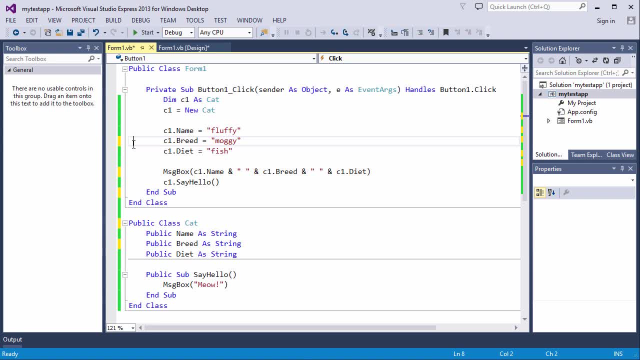 for example, I might have a calculate pay method or a method that will save the employee details into a database. We'll see some more realistic examples in later videos. OK, so let's take things a stage further here. I want another cat. 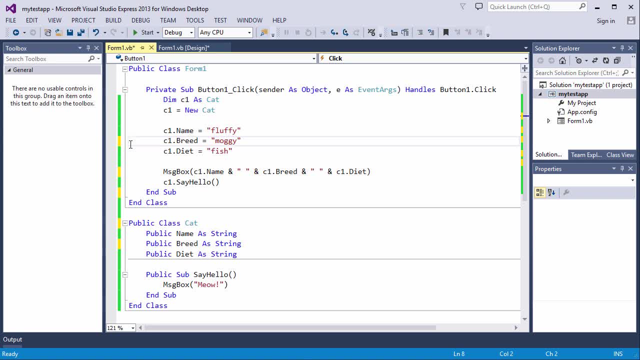 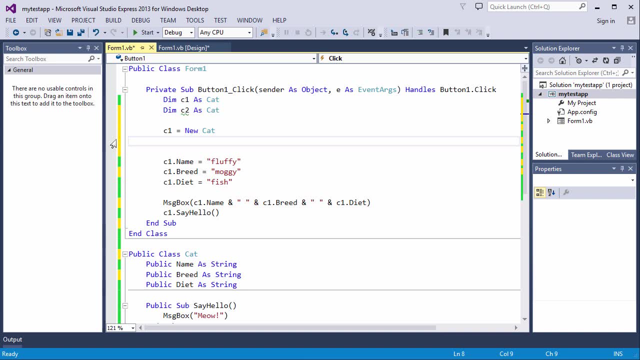 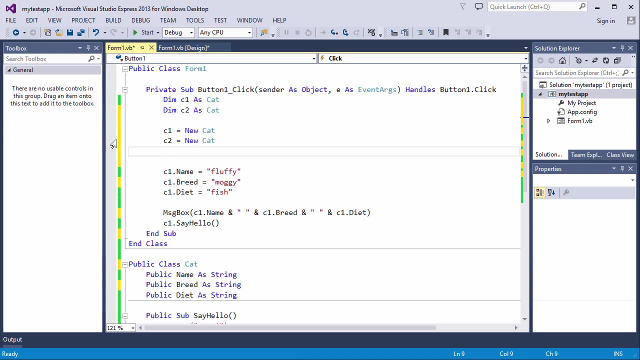 So I'm going to declare another variable of type cat And I'm going to bring this cat to life as well. I'm going to create an object from the class. When this line of code executes, I'll have a second cat, Right, let's set some properties. 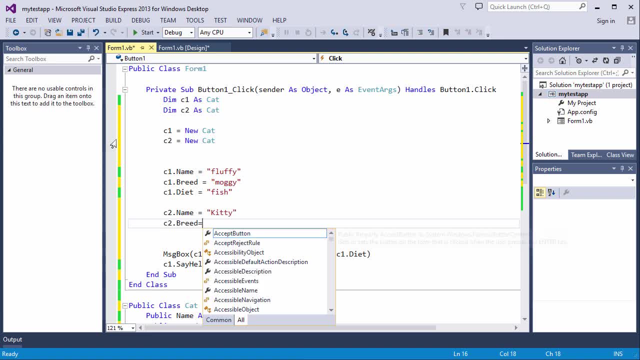 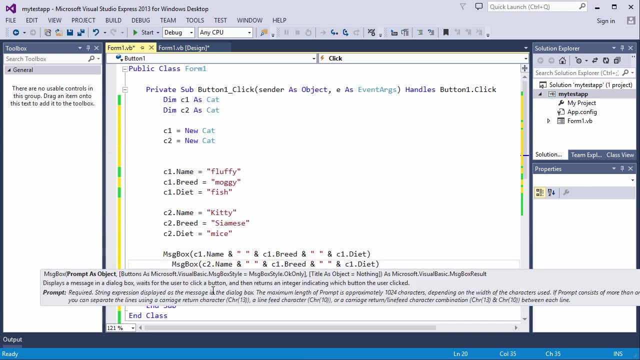 Yeah, OK, I don't suppose people feed their cats mice. but that'll do for now, And let's output details of this cat as well. I'll just do some copying now, I think. 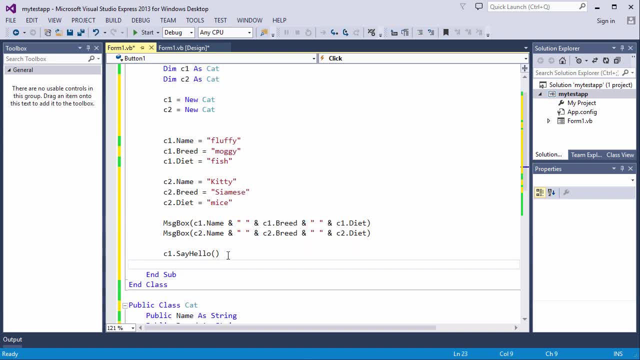 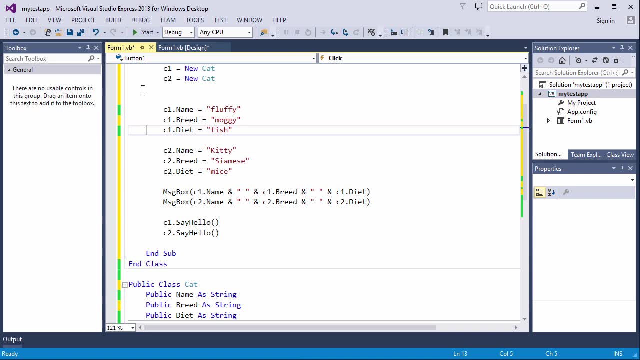 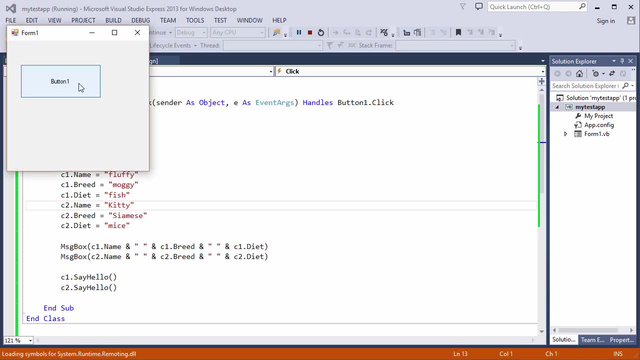 And let's call the say hello method for my second cat. OK, let's see what we get this time. There's my first cat, Fluffy. There's details of my second cat, kitty. there's my first cat saying something, oh, and there's my second cat saying exactly. 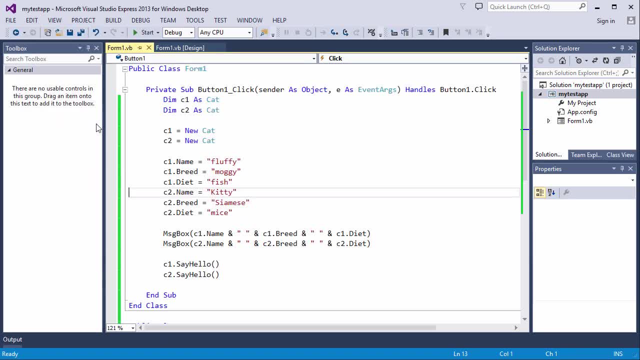 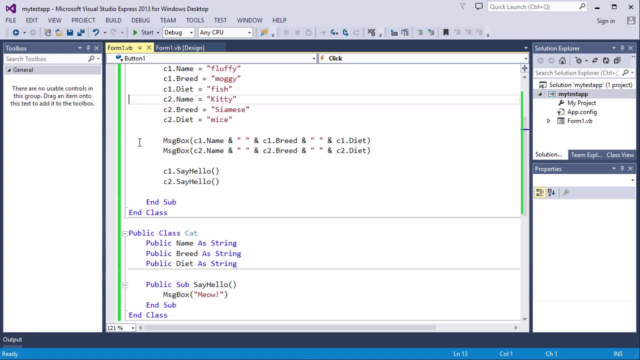 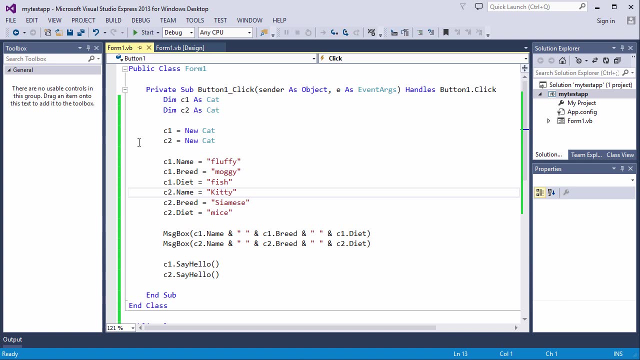 the same thing. Alright, so I've got two cats which I've created using the same class, And of course, I can have as many cats as I like, which will all be instances of the same class. So, strictly speaking, an object is an instance of a class. There's just a couple. 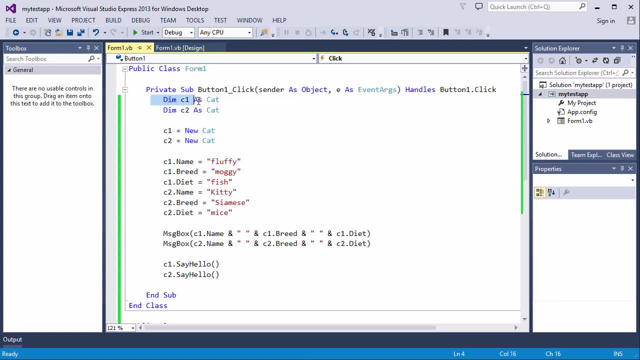 more things I want to show you very quickly. First, I'm going to combine my declaration with the code that creates a new instance of the cat class, like this: Dim C1 as new cat, which means I don't need this line. I can do the same here as well. Dim C2 as. 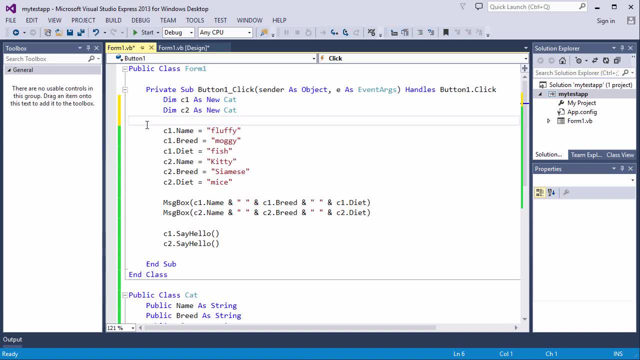 new cat. Alright, so I've just got rid of a couple of lines of code. That's fine, but it begs the question: why did I not just use two lines of code in the first place? Sometimes you want to keep your variable declarations. 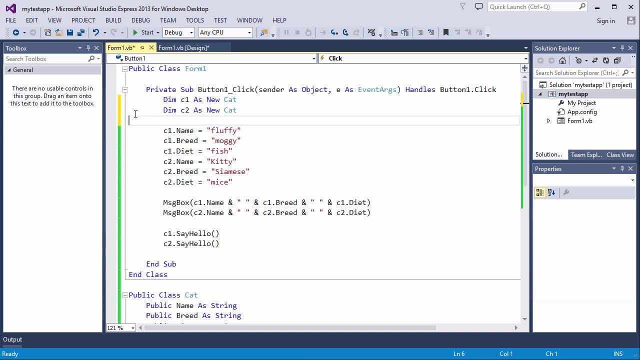 together at the top of the program. but you might want to delay the creation of an object until as late as possible, which is why I would use two lines of code instead of one to create a new instance of the class. OK, now I want to release the memory that was. 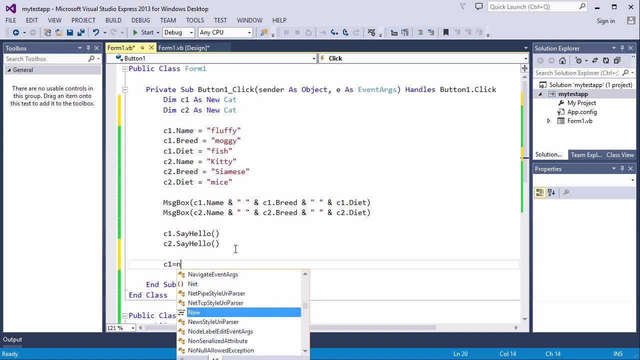 being used by these objects. And you can see what I'm doing here is I'm setting the object variables to be equal to nothing. Now, the truth is, when this program stops running, the memory would be released anyway. The VBNET runtime engine, the so-called NET framework, has a little subsystem called the. 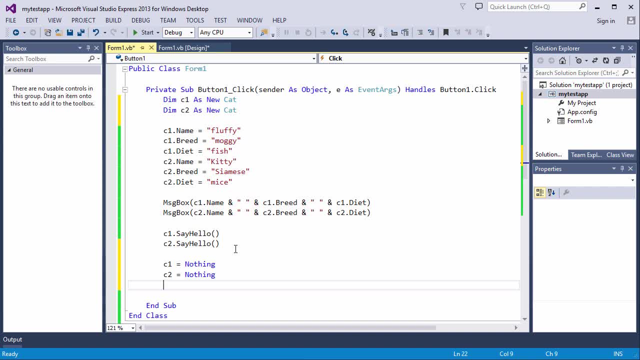 garbage collector, which will free up that memory anyway. But those two lines of code could be used anywhere in the program to release that memory. if, for example, I want to free up some resources early, So I always put them in at the bottom of my program as a matter. 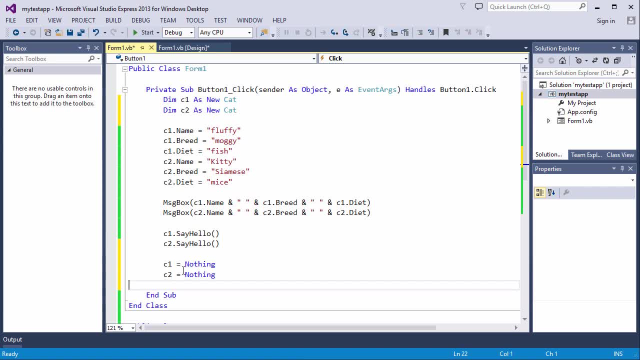 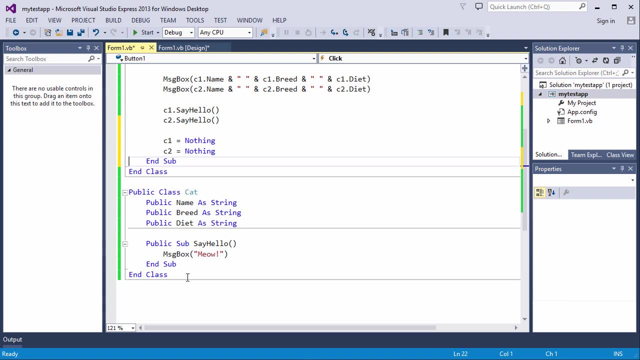 of course, in control Right, so let's just refine our definitions here. An object is a thing from the real world, It's an entity that we want to store and process data about, But it's also an instance of a class. A class, on the other hand, is the code that defines.